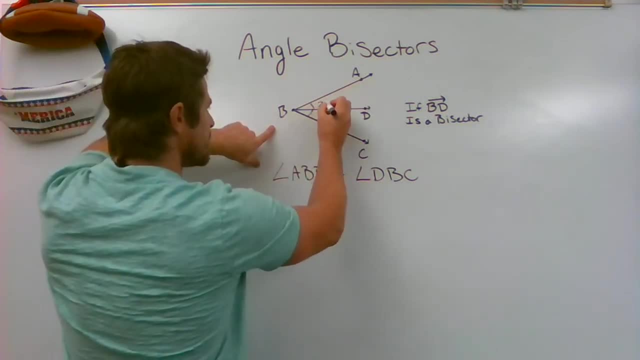 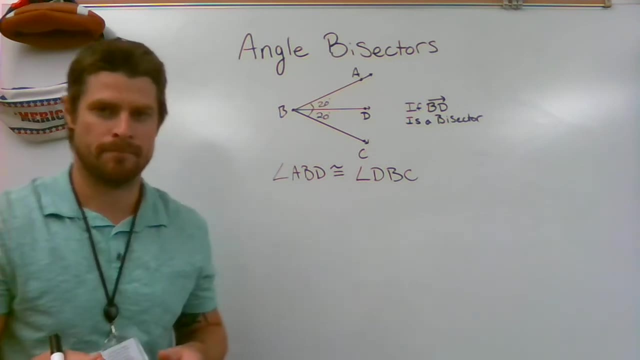 well, this 40 degree angle would break this into a 20 degree and this into a 20 degree. They're going to be equal. They're going to be the same, All right. so all it's doing is taking the large angle, cutting it. 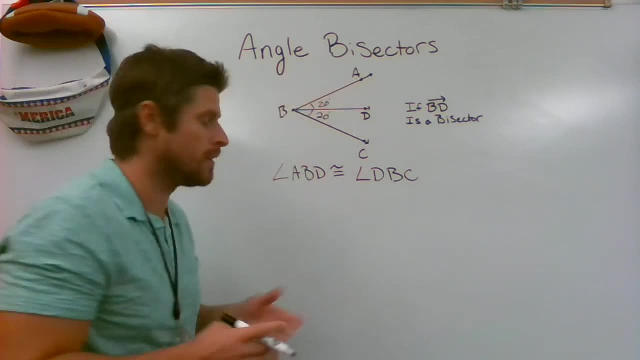 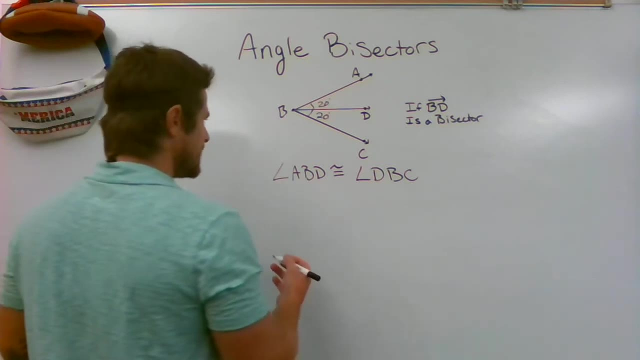 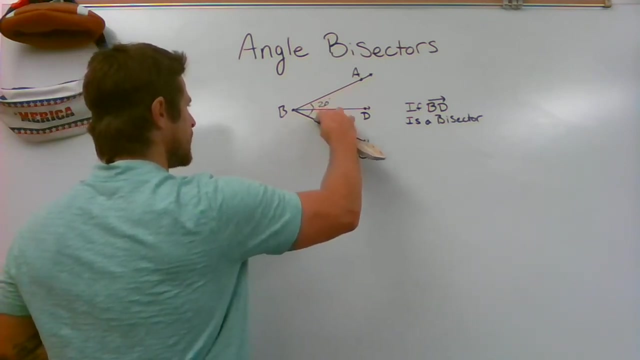 into two equal angles, cutting them in half, All right. so how are we going to see problems in a geometry course? What are those going to look like? Let's say we are told for this problem exactly, or for this picture diagram, exactly that angle. 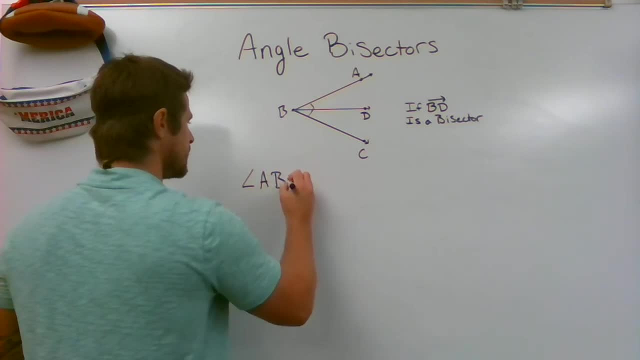 ABD and I always. one thing I always like to do a little tip is I'll read it and then I'll kind of do a quick scan with my finger over the top. So I'm talking about this angle and if I'm told that, 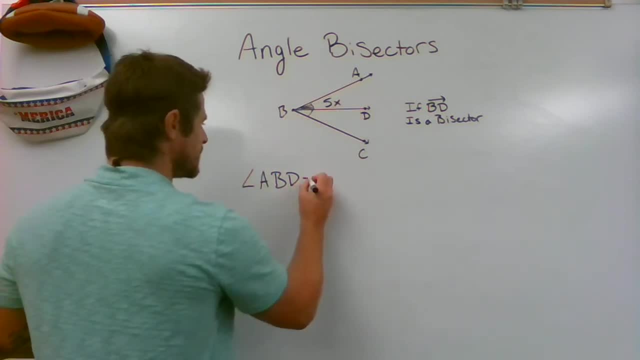 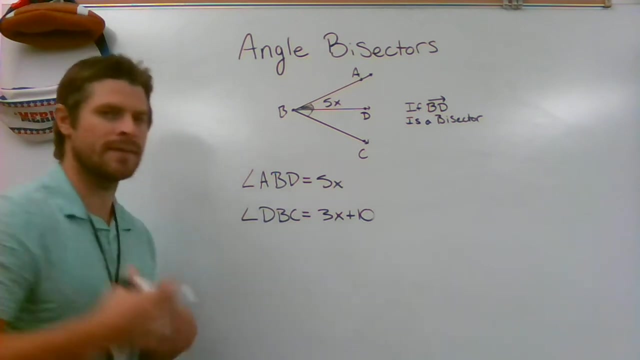 that is 5X. so if I'm told angle ABD is equal to 5X and then I'm also told that DBC angle DBC is equal to 3X, 3X plus 10.. Let's say I'm given that information and I'm also told BD ray BD is a bisector. 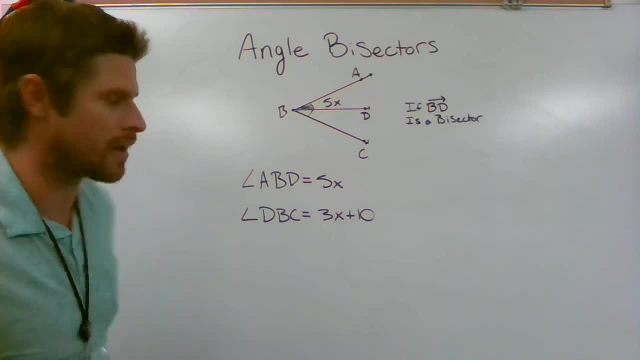 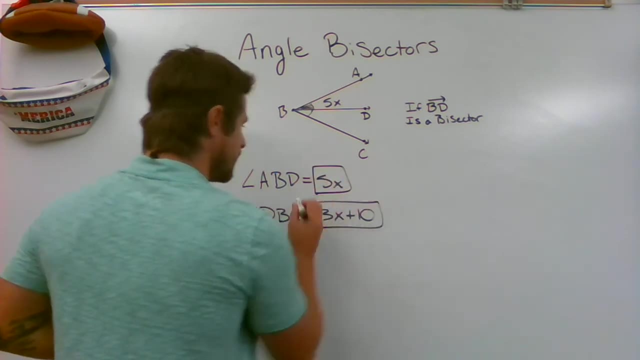 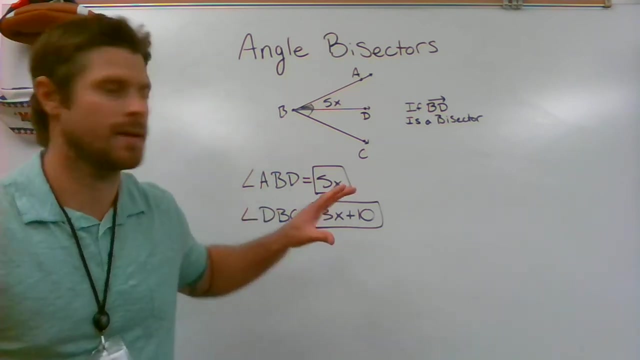 Well, I can figure out exactly how large these angles are by using algebra. All right, I'm going to take this expression and this expression and I have to ask myself: what do I know about those two given angles? I know they're the same. I know that this angle is the exact same angle. 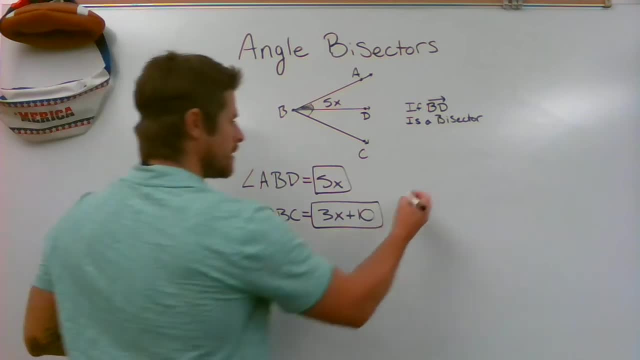 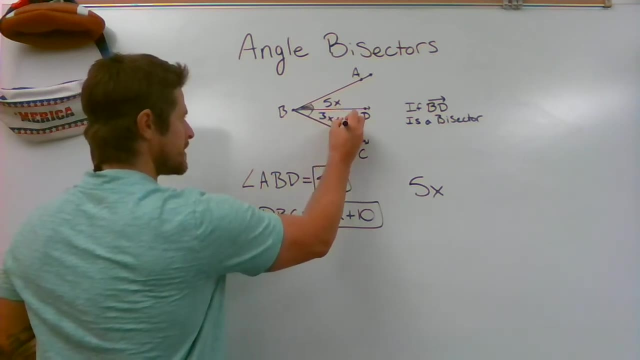 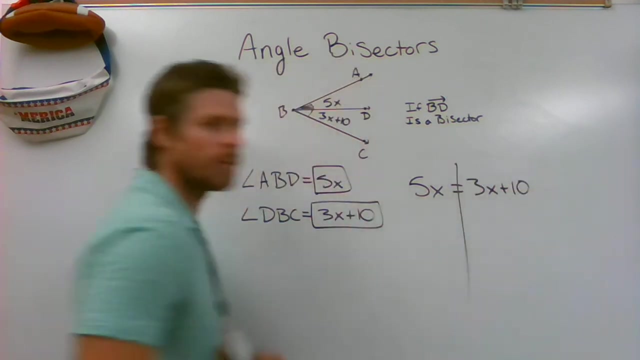 I know that this angle is the exact same as this angle. How do I say that? in algebra, That equal sign says that 5X is the same as 3X plus 10.. It's equal to 3X plus 10.. Now we go back one year from. 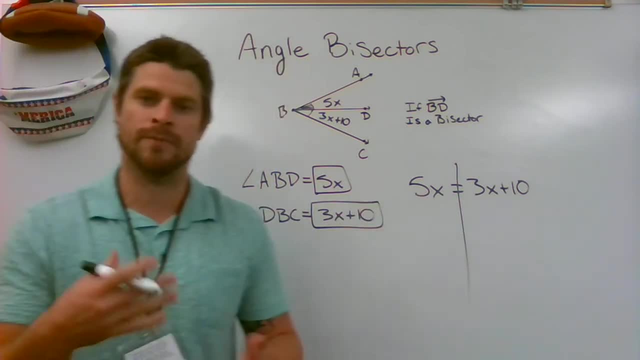 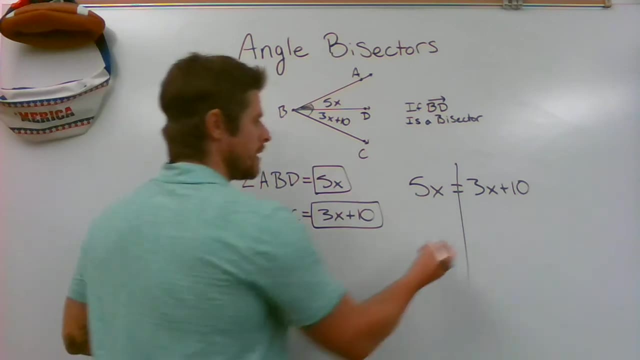 geometry. back to algebra. We do our algebra. We figure out what X is. Once we know what X is, we can plug it in and it will tell us exactly how big each angle is. So how do I do Variables on both sides? I'm going to have to subtract 3X from this side. Subtract 3X from this. 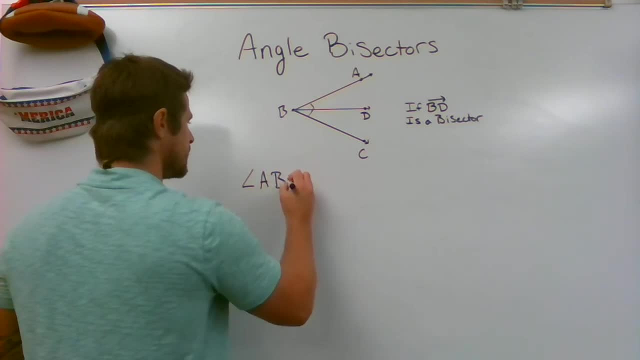 ABD and I always. one thing I always like to do a little tip is I'll read it and then I'll kind of do a quick scan with my finger over the top. So I'm talking about this angle and if I'm told that, 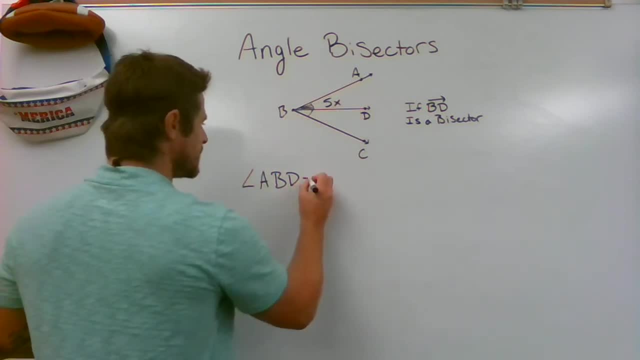 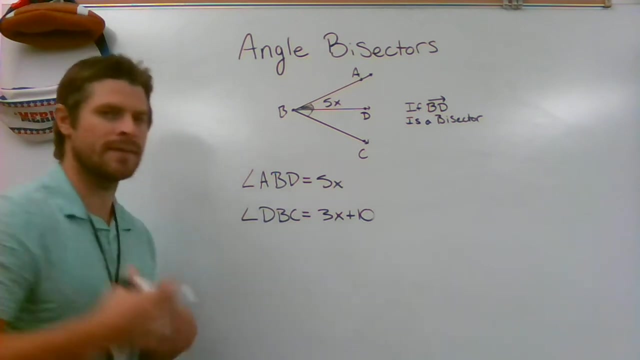 that is 5X. so if I'm told angle ABD is equal to 5X and then I'm also told that DBC angle DBC is equal to 3X, 3X plus 10.. Let's say I'm given that information and I'm also told BD ray BD is a bisector. 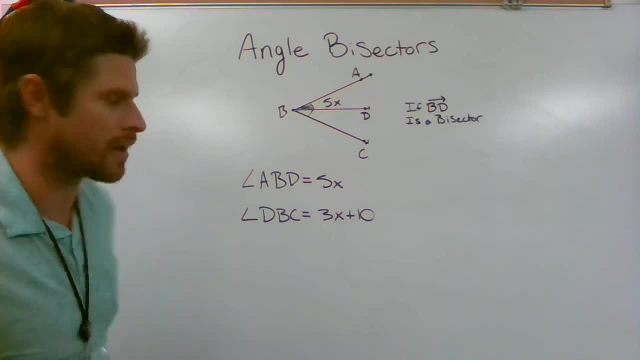 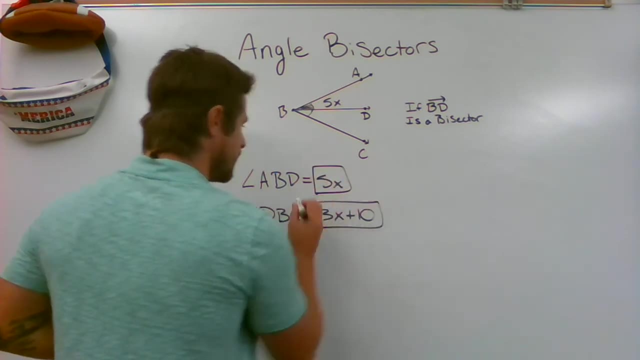 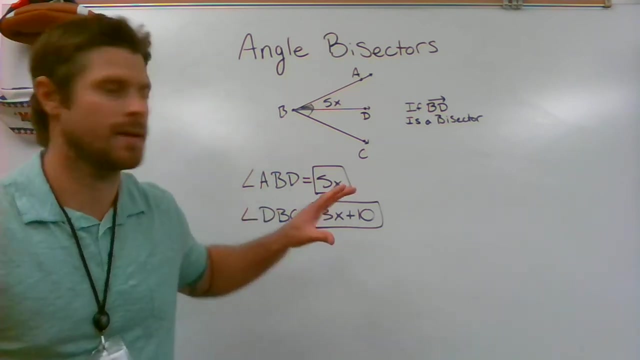 Well, I can figure out exactly how large these angles are by using algebra. All right, I'm going to take this expression and this expression and I have to ask myself: what do I know about those two given angles? I know they're the same. I know that this angle is the exact same angle. 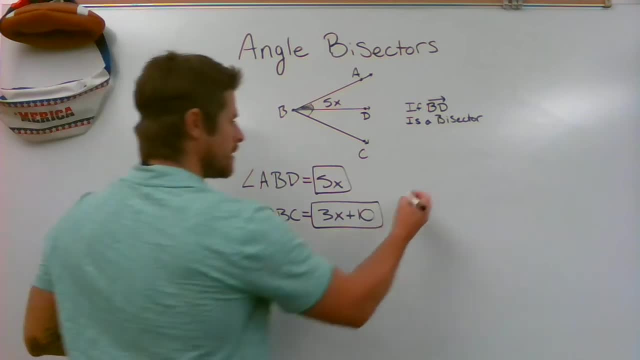 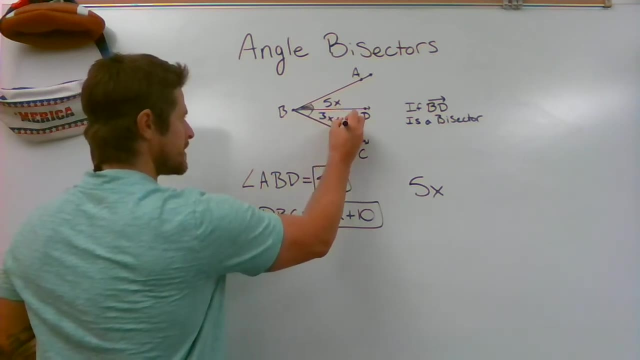 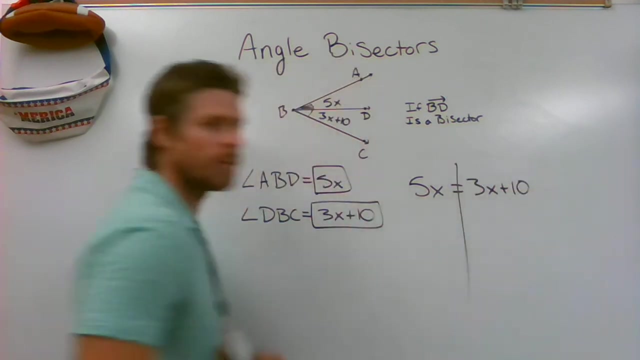 I know that this angle is the exact same as this angle. How do I say that? in algebra, That equal sign says that 5X is the same as 3X plus 10.. It's equal to 3X plus 10.. Now we go back one year from. 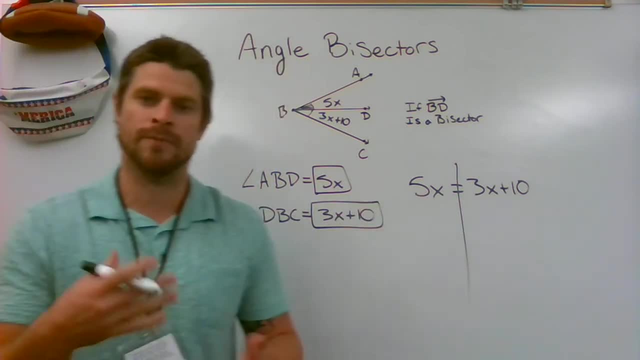 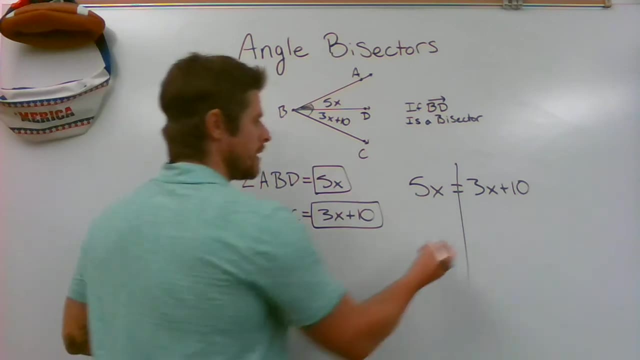 geometry. back to algebra. We do our algebra. We figure out what X is. Once we know what X is, we can plug it in and it will tell us exactly how big each angle is. So how do I do Variables on both sides? I'm going to have to subtract 3X from this side. Subtract 3X from this. 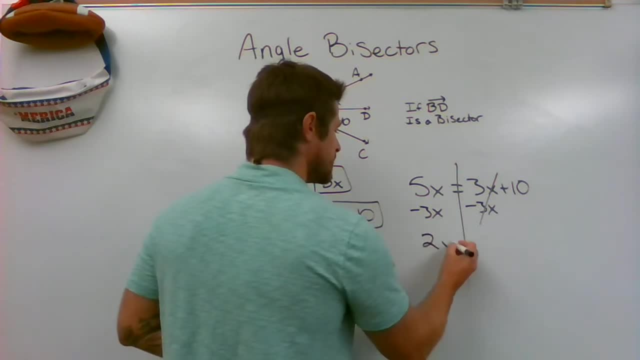 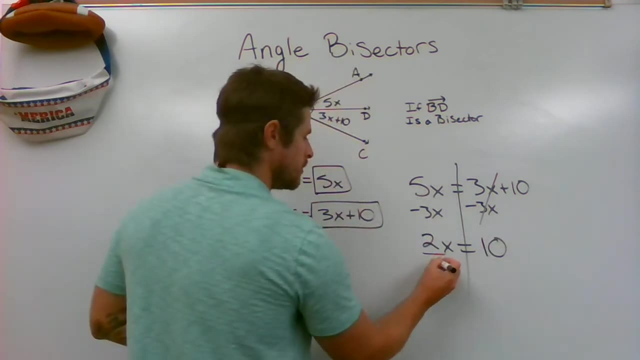 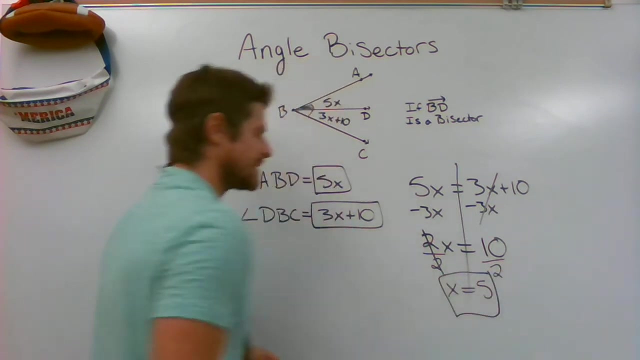 side Like terms. Now I have 2X and it's equal to the only thing that's left on the right side of 10.. Divide by 2 to cancel out the 2.. Divide by 2. X equals 5.. Okay, I know what X is. Do not jump. 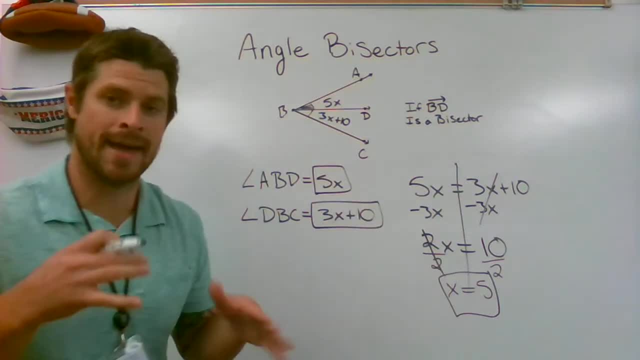 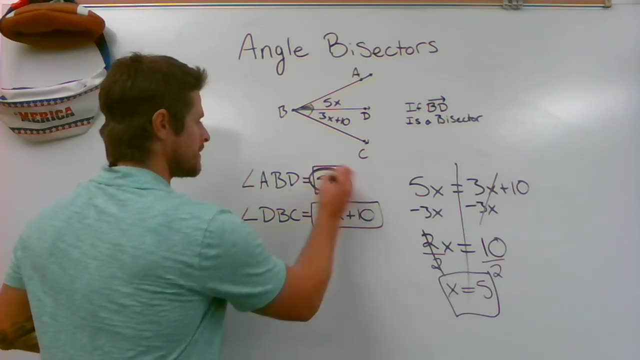 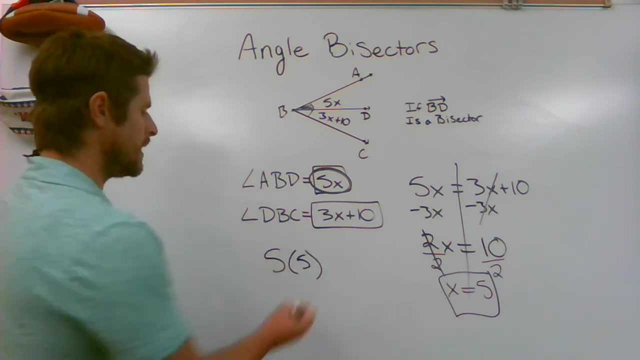 up here and say: oh, the angle is 5 degrees. It's not 5 degrees, X is 5.. X is 5.. The angle, remember, is 5X. So you want to say 5 times 5, and what you would get is an.